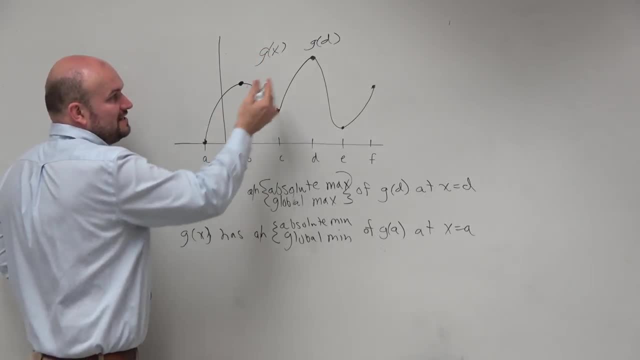 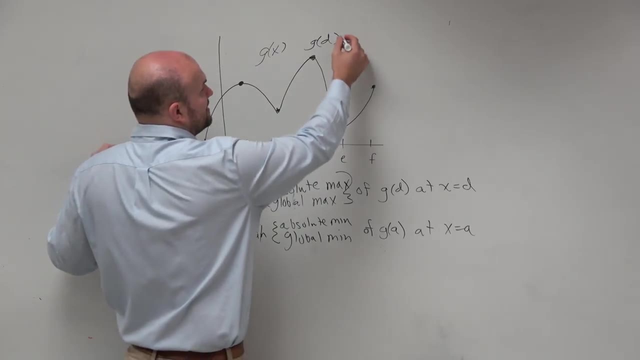 or like your y value, is the absolute highest point. So the definition of a maximum or a minimum- let's just talk about a maximum- is that anything of that a is going to be greater than or equal to f of x on our interval. 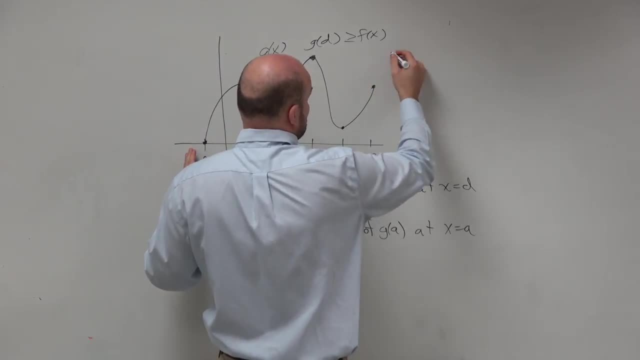 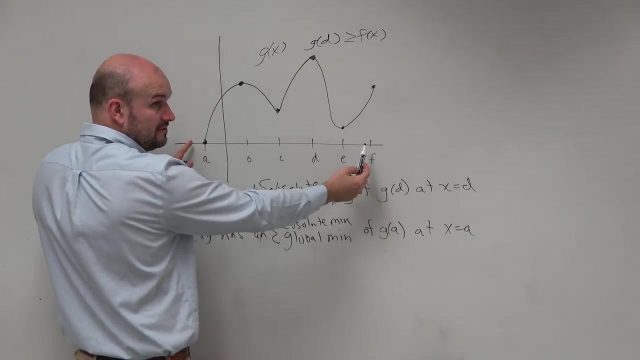 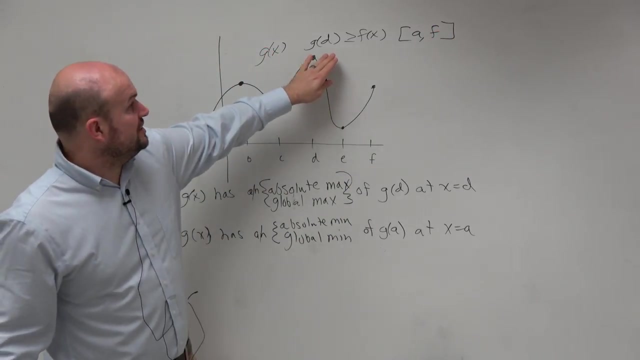 So if we look at this interval, we can see that this closed interval really doesn't matter on our interval. But on this interval of this graph which is from a to f, that's like our interval here. the value of g of d. 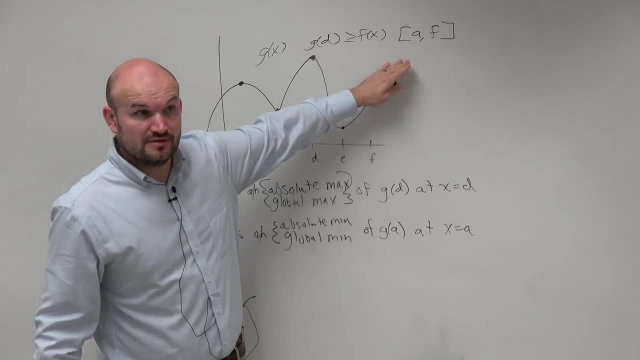 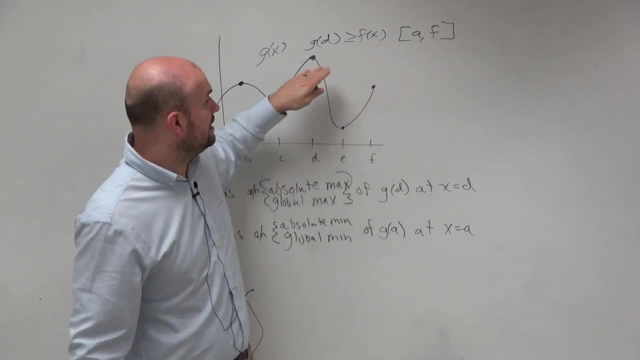 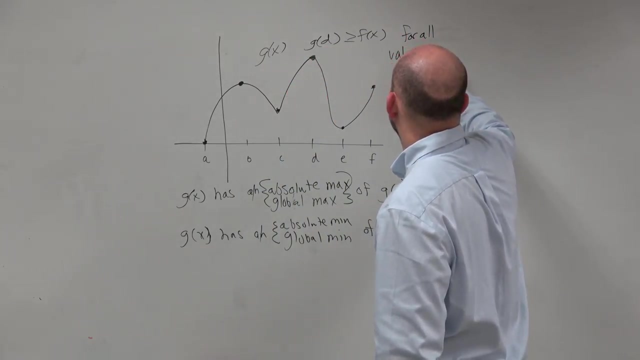 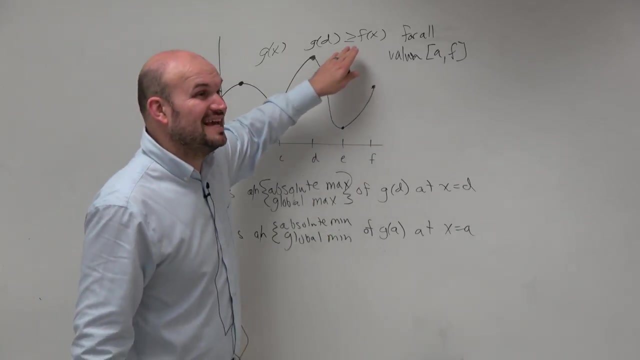 is greater than or equal to f of x for all values, for all x values on the interval from a to f. Do you guys agree? Do you guys agree? That's what makes that- I'm going to say this So- any output value, that is absolutely the highest. 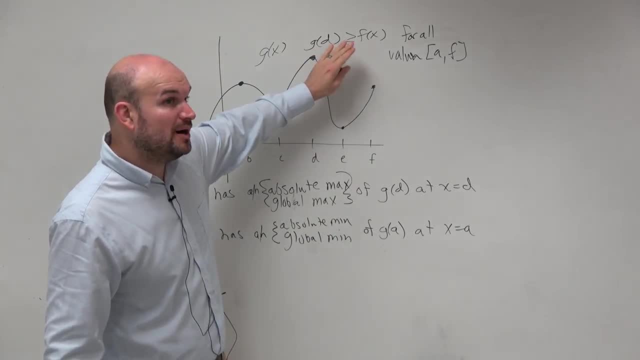 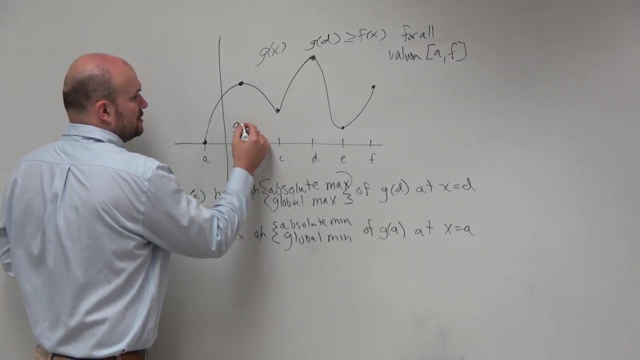 Now it could be greater than or equal to right. We could have more than one, but that is going to be your highest value. Then, when we're talking about the minimum, it's kind of like the same thing: g of a is less than or equal to f of x. 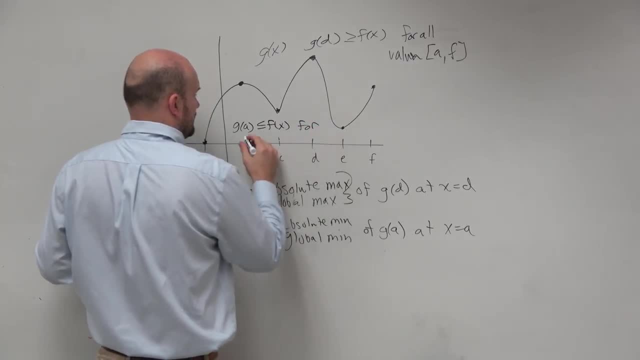 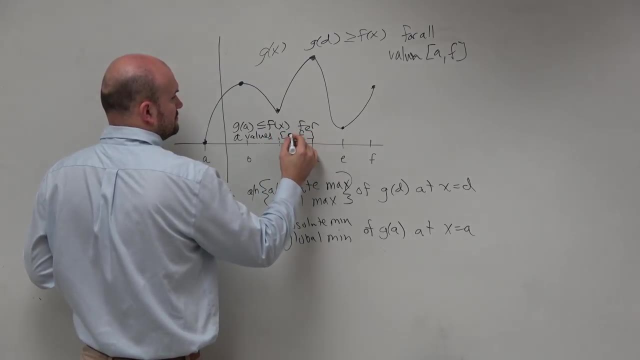 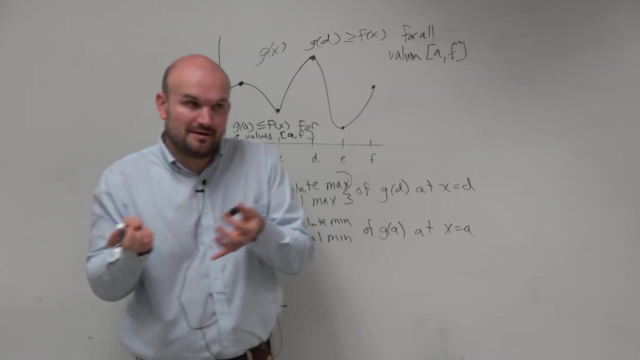 g of a is less than or equal to f of x, for all values on the interval a to f. Now, this is obviously a closed system. That's included and that's included. But the basic thing, when we're looking for an absolute minimum, absolute maximum, 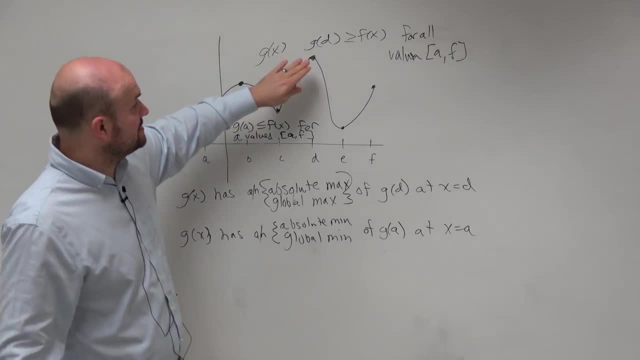 what we're looking for is we're looking for the value that is going to be obviously the largest, Because if you put any point to the left or any point to the right, it's not going to be as high as g of d. 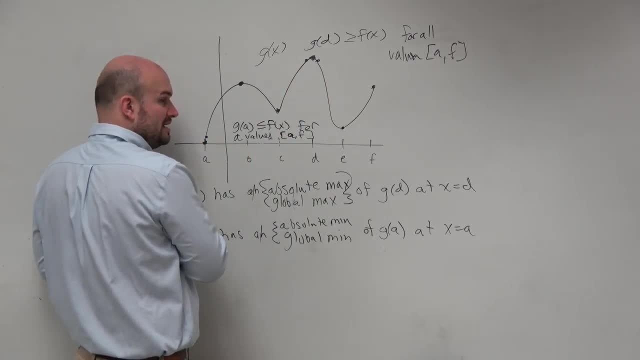 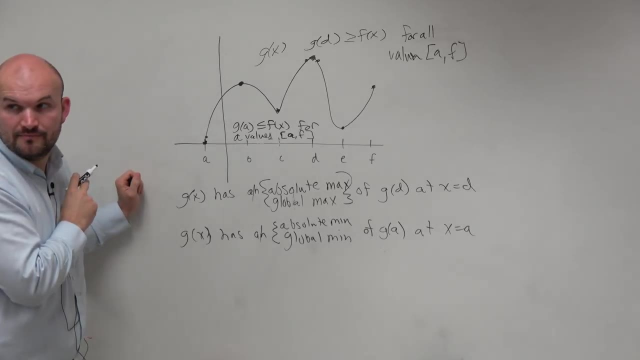 Do you everybody agree? Any point to the right of g of a is obviously higher than what g of a is. So g of a is the absolute smallest that we have. Everybody agree there. So just make sure you guys understand at least. 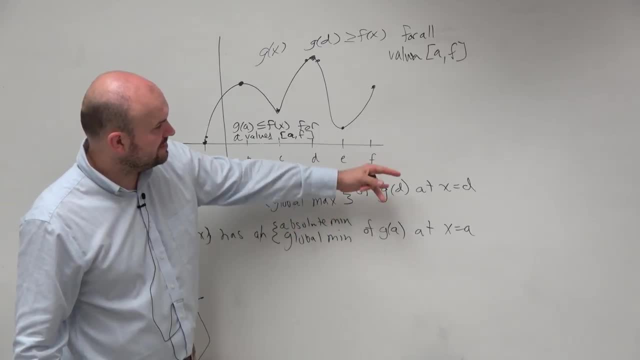 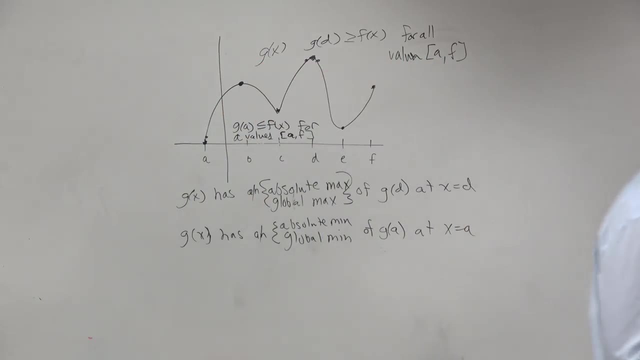 these are interchangeable terms, absolute and global- And then obviously we talk about the values, which is the max or the min, but then also where those values occur. So that's absolute.